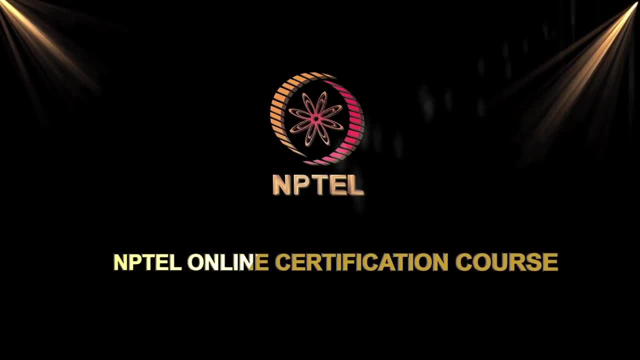 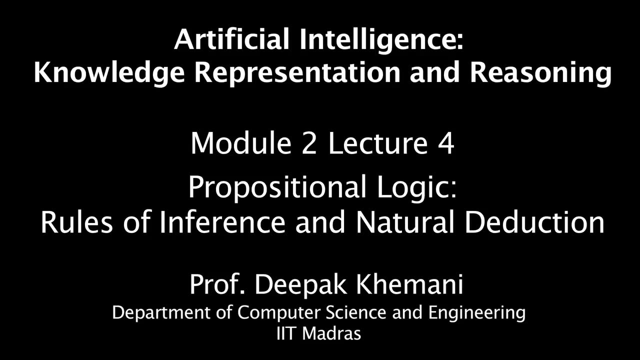 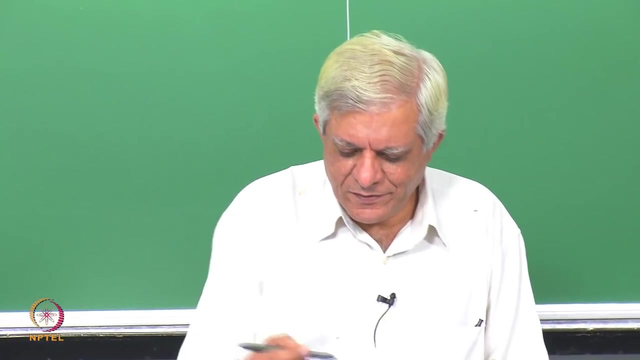 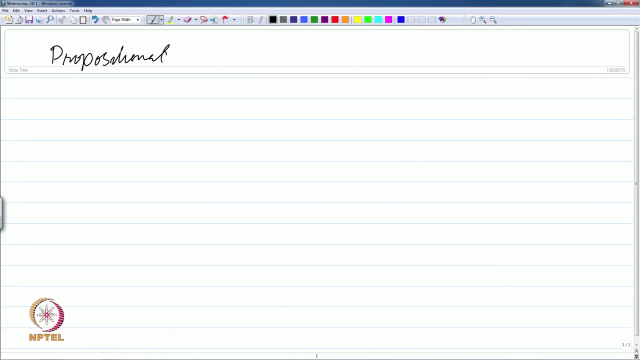 So let us continue our study of Propositional Logic. So, to do a very quick recap, we first looked at the syntax, and in the syntax, once you define an alphabet, you get a language. So the alphabet includes, if you remember things. 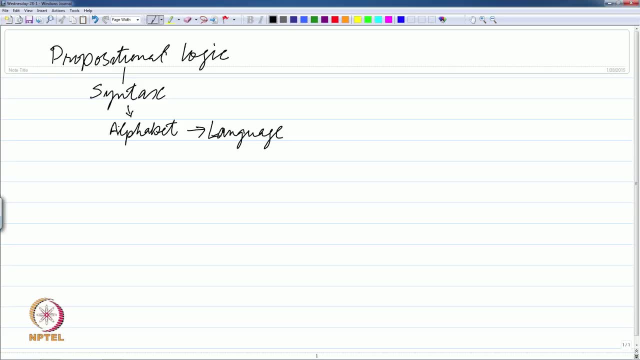 like connectives and propositional variables and so on, essentially. So a language is basically a set of sentences and the alphabet is essentially things like AND OR NOT, P, Q, R, without going into details, these are the kind of things that we had. 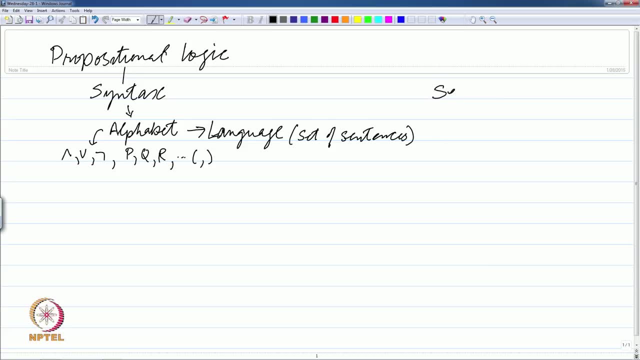 And then we have semantics. So, as far as Propositional Logic is concerned, by semantics we mean truth, functional semantics. We defined the notion of truth, values and we saw that, Ok, These are. there are 3 kinds of formulas or 3 kinds of sentences in any language. One: 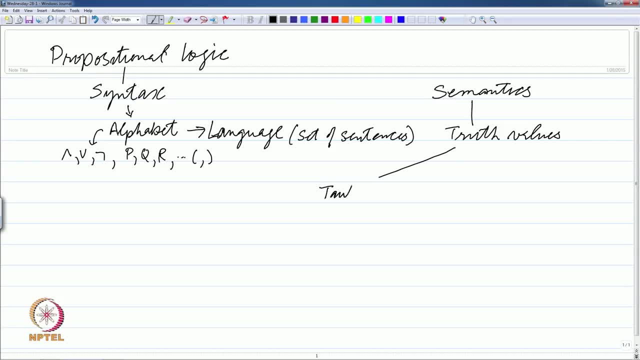 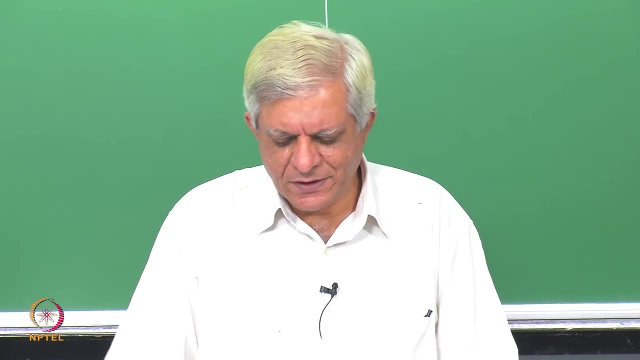 is tautologies. these are sentences which are always true, and we say always true, we basically mean they are true for any valuation of the atomic propositions. So, whatever the atomic propositions are- P, Q, R, S, P and so on- Whatever valuation we give to them, 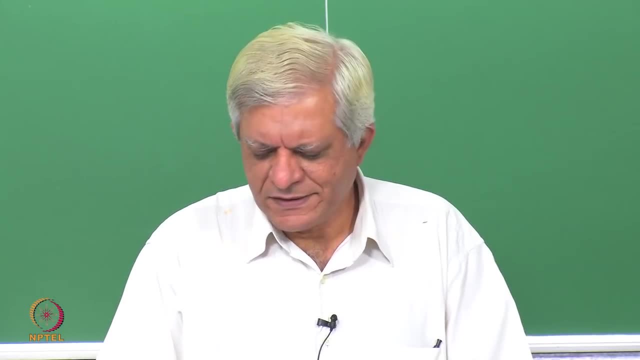 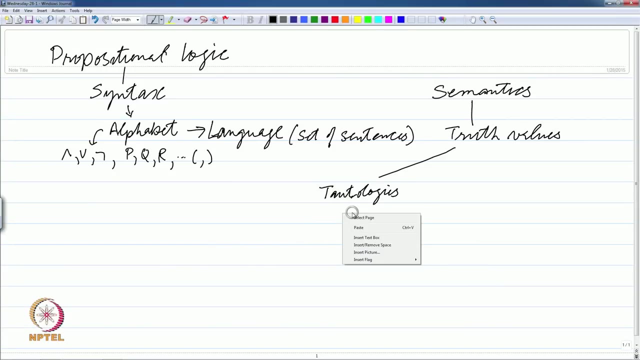 which means true or false. the phrase is the same. girl should not be used inöttler-ter anterior. true or false, these sentences will always be true. and then trivial example of that was p or p or not p. Then we have sentences which are contradictions. 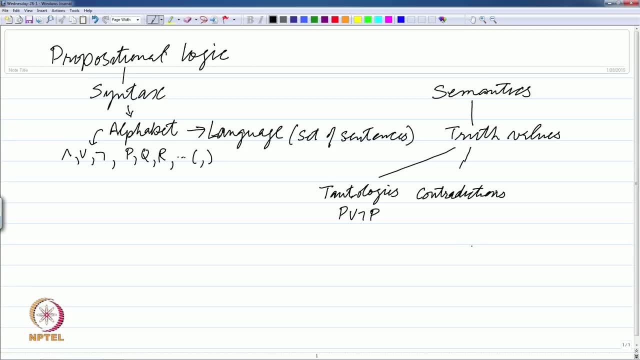 and these are sentences which are always false, which means that any valuation that you choose, they will be false. and an example of a contradiction is this sentence, which is a negation of the tautology that we have seen. essentially, I have, I have particularly chosen this: 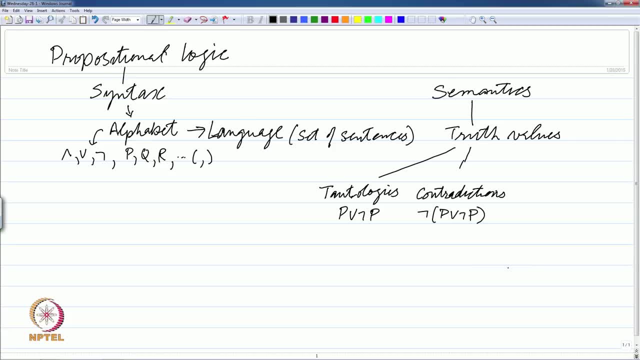 example, because there is this relation between contradictions and tautologies, that if you have a tautology and you put a negation sign before that, it will become a contradiction and vice versa. So in this case we have taken a tautology, p, or not. p put a negation. 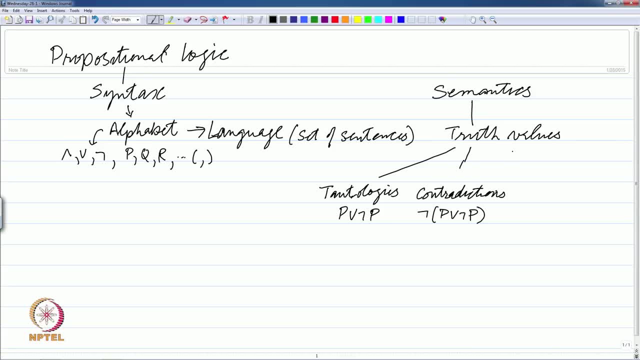 sign in front of that And it is become a contradiction. and the third kind of sentences are contingencies. and by contingency we mean that the truth value of the sentence depends upon the valuation that you are choosing. So a sentence like p implies q, for example, will be true if for 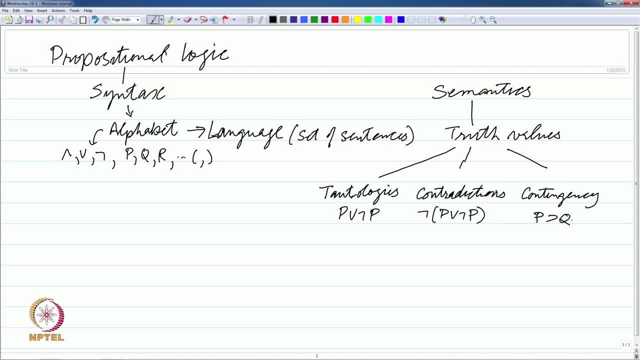 example, you choose, p is equal to true and q is equal to true. but it would be false if you choose p is equal to true and q is equal to false. essentially, So it it is. it is truth. value is not independent of the valuation. it depends upon the 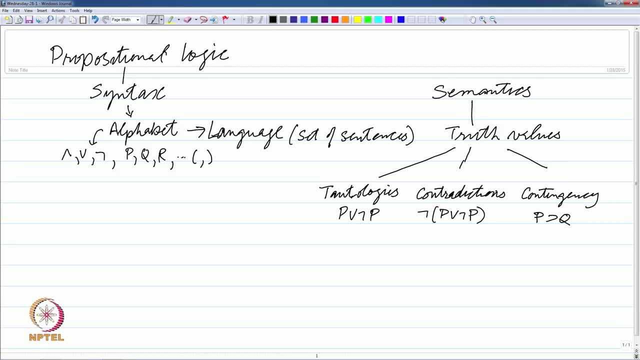 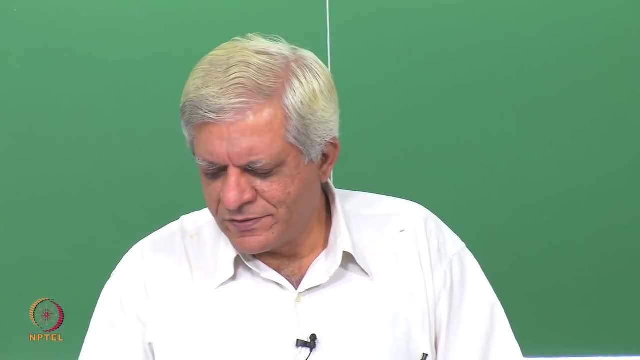 valuation essentially. So we would be more interested in tautologies and contradictions, because we are interested in proof systems. We want to show that whenever certain formulas are always true, we have a way of reaching to those formulas. So before we do that, so when you talk about contingencies, we essentially talk of satisfiability. So 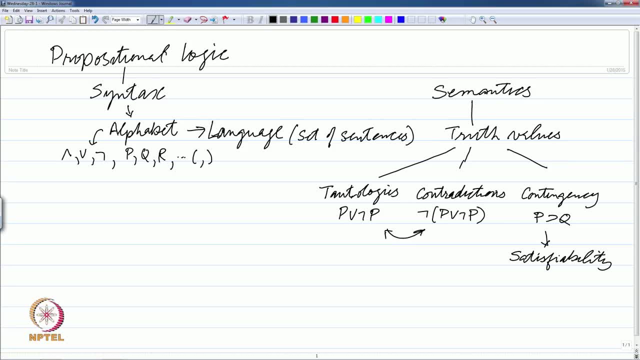 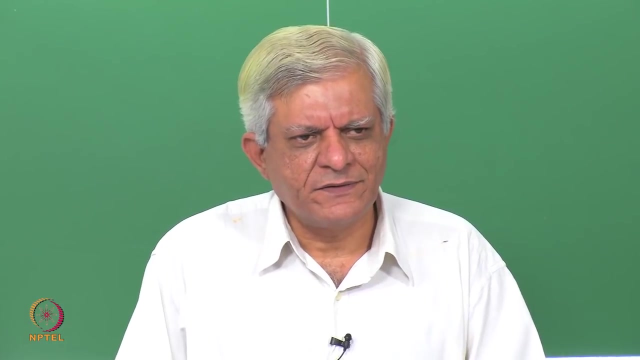 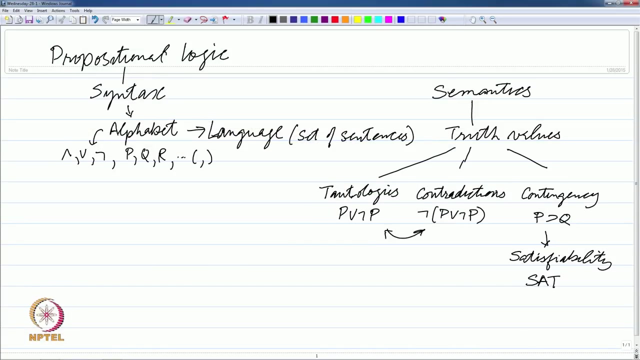 you would find that you are familiar with contingencies, but there areMarillyes' and Sarsour keshy what we talk about. Then we define the notion of entailment. So if you remember the, 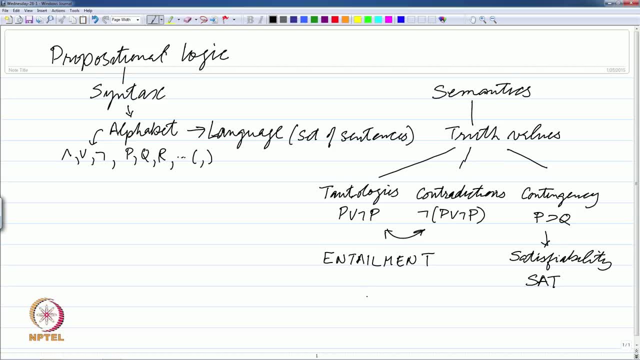 notation. we said that a knowledge base, K B, which is basically a set of sentences that are given, entails a sentence alpha whenever alpha is necessarily true as long as the K B is true. So whenever K B is true, alpha will be true, and this is the notion of entailment. essentially Correspondingly at the syntactic level, we 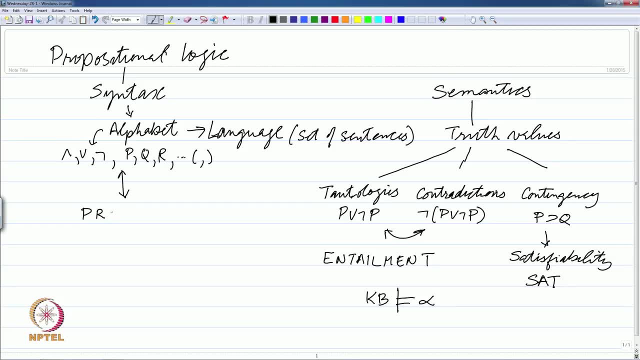 have this notion of provability or the notion of proof, And that is the concept that we are going to be exploring in the in most of this course essentially, And we write that a knowledge base proves, or you can prove a sentence alpha given a knowledge base. essentially. 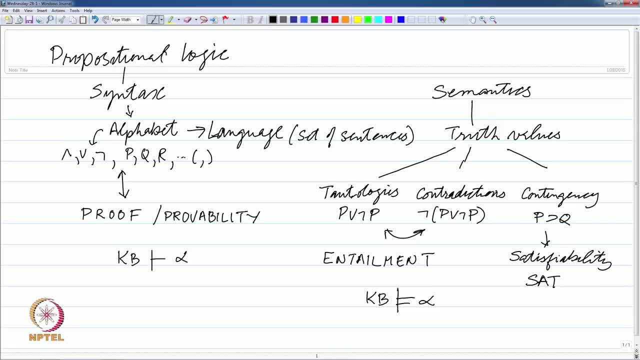 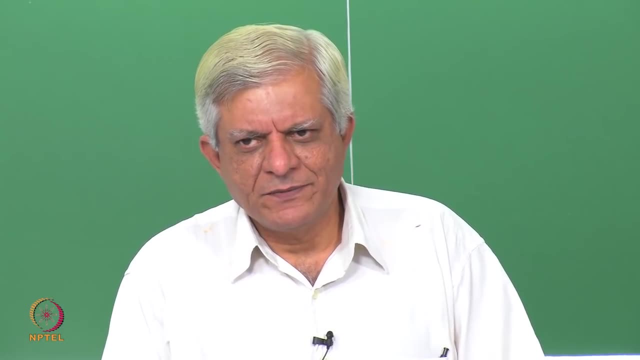 So essentially we are interested in that kind of a logical machinery where provability implies truth or entailment, and entailment implies provability, which means we want to be able to prove all true formulas and we want to be able to prove only true formulas. 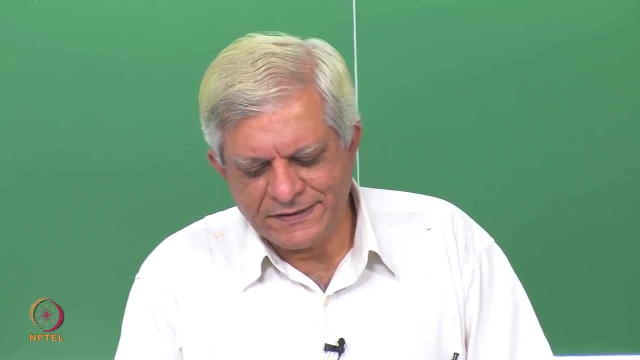 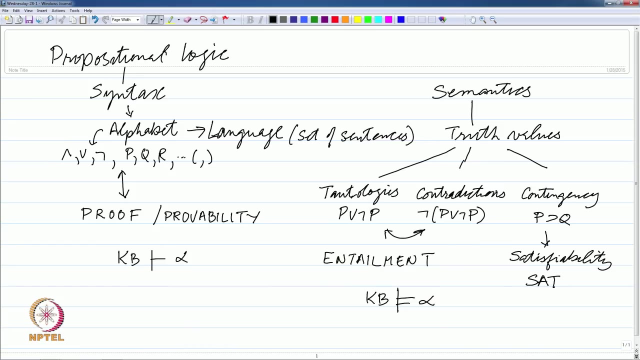 Once we have such a machinery, we can actually throw away the notion of semantics and we can just work with the syntactical machinery, which is the proof machinery, essentially Now a proof. for a proof system to work, we need a language that the syntax gives us. 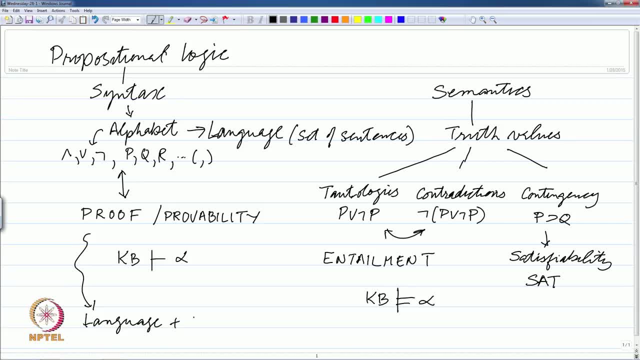 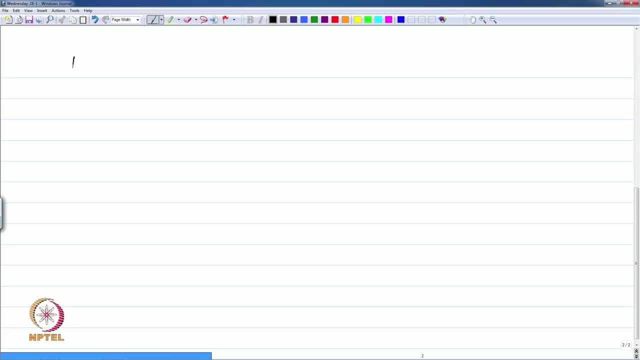 plus, we have rules of inference. So let us look at proof systems. So let me start with an example rule, The rule that we have been…. We always start with more or less whenever we look at logic, And that is the rule of modus ponens, which. 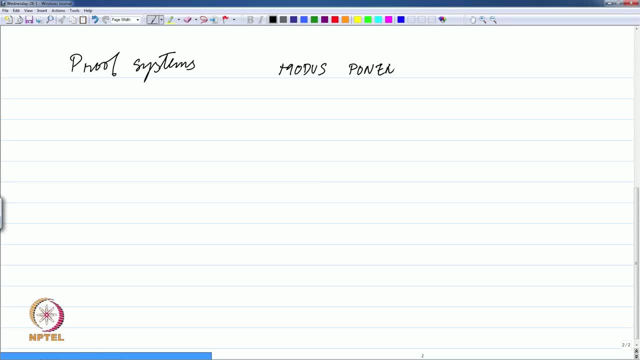 we have seen earlier, And the rule is written most commonly as p and p implies q And you then q. So the sentences above the line are the given or the antecedents, and the sentence below the line is the consequent or what you derive essentially. We also write this if: 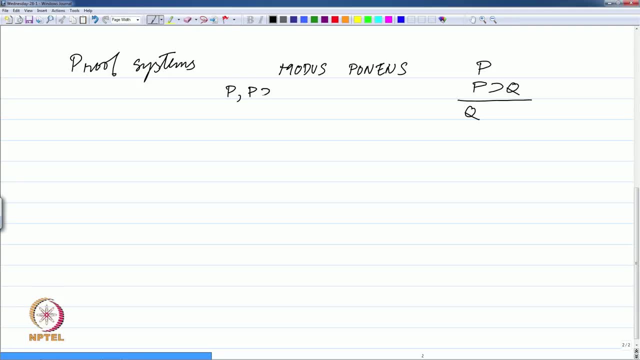 you remember, as p, comma, p imply q, and we use this notion, that this symbol that we have is q, And this rule we will call as m p, which is the short form for modus ponens. essentially Now, the first thing to emphasize, which I 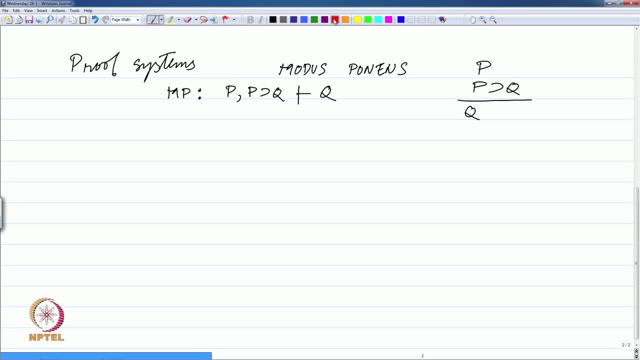 have done earlier also, but just to repeat that p and q are propositional variables. It means you can plug in any sentence in place of p or q, So for instance. so what this defines is only the form of the argument. So I could have written something like this: 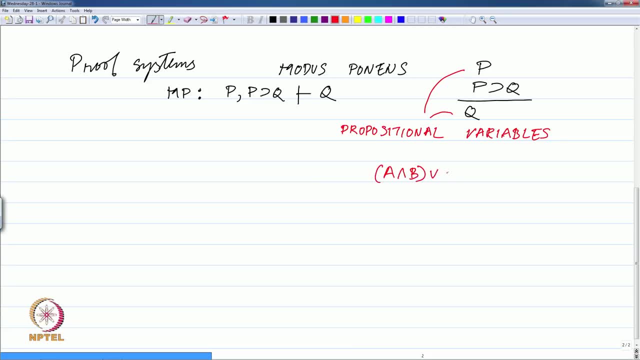 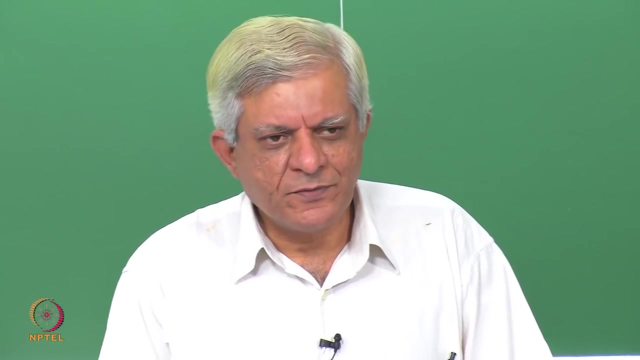 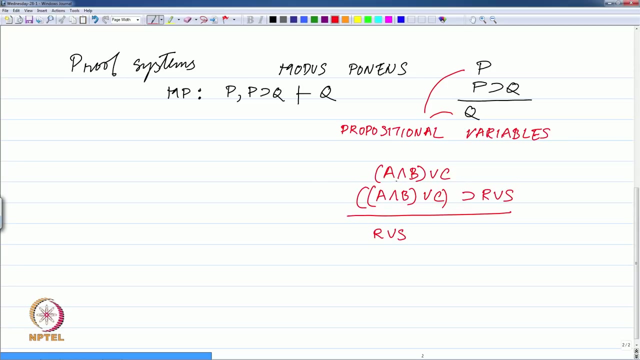 a and b or c, And then I can write: a and b or c implies r or s … S, and from this I can define R over S. So if I do this, I am still using the rule of modus ponens, because essentially what I have is something, a sentence of any kind, which 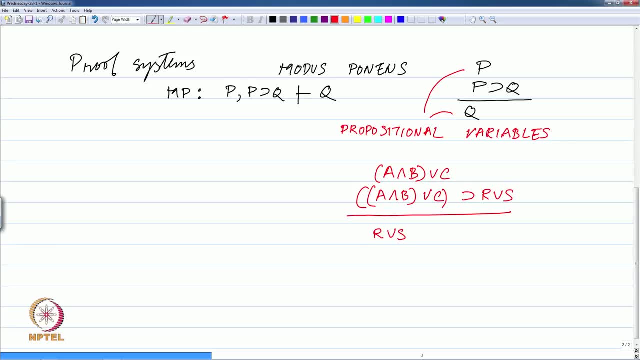 in the original notation we said p, but in this particular example that the sentence is a and b or c. and then we have another sentence which says that a and b or c implies R or S, and from there, if we can add R or S, then 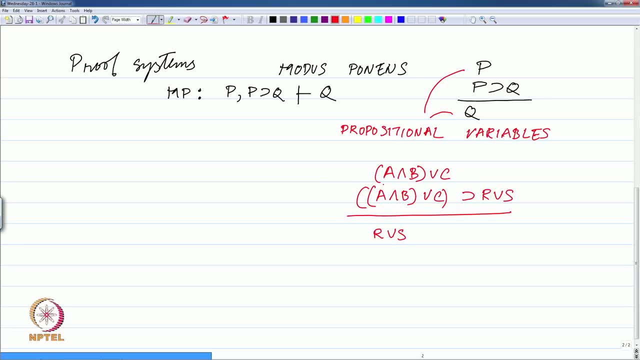 we can. this is also an instance of modus ponens. So this is just to emphasize the fact that when we say p and p implies q implies q. these are propositional variables and you can plug in any sentence. it does not even have to be. 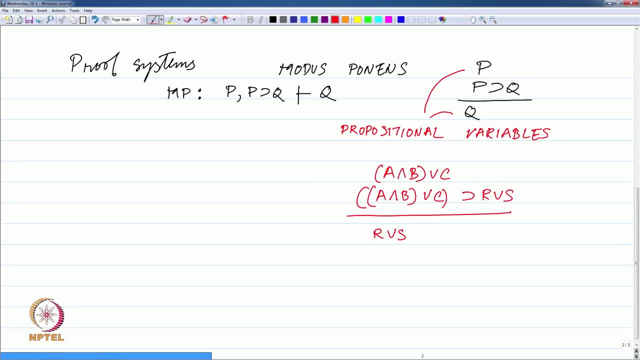 in propositional logic, it can be in first order logic or any modal logic Or any other logic set. you know that one may, so really we should write is something like this: that if your sentence 1- whatever the sentences in fact in any language, and if you have 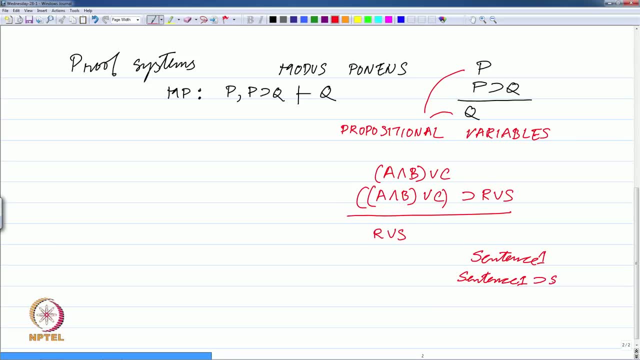 another sentence which is of the form: sentence 1 implies sentence 2.. Then we can infer sentence 2.. So this is a rule of modus ponens, and we saw that there are other kind of rules. So what do we mean by rule of modus ponens? that it is a form of argument. 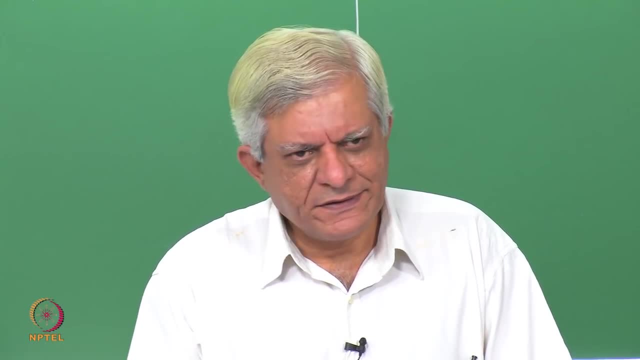 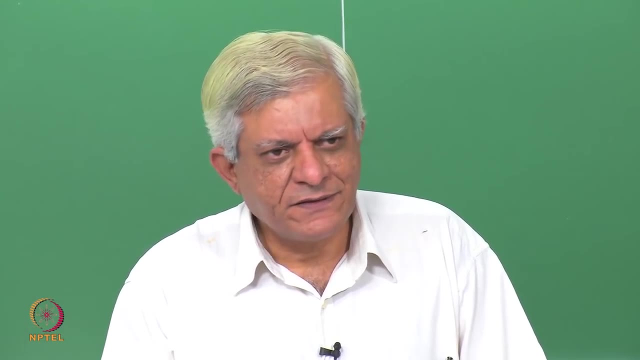 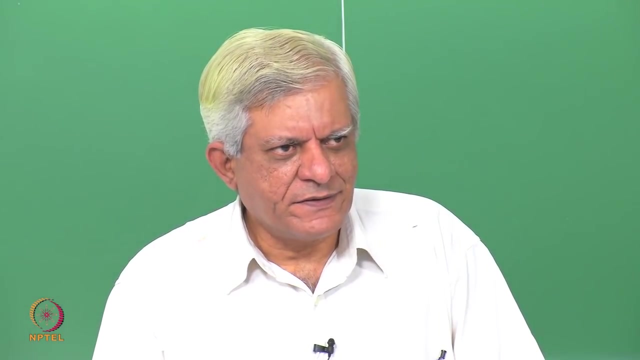 that we are willing to accept, which says that whenever we have 2 sentences which match this pattern, that one of the sentences of the kind p and the second sentence of the kind p implies q, then we can make an inference of the third sentence, which is q. essentially. 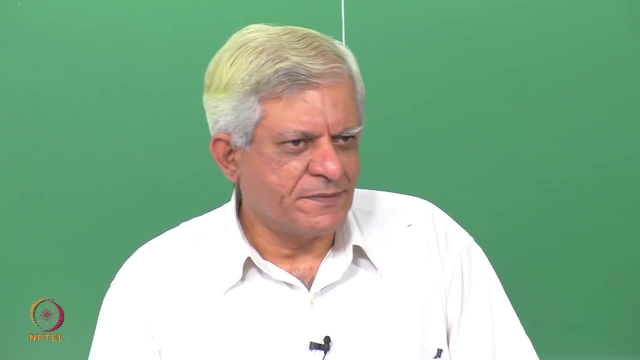 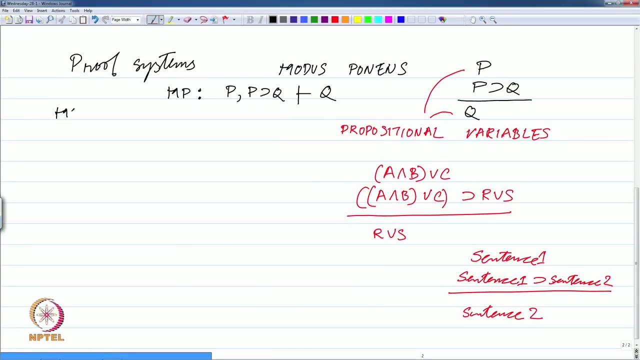 Whenever this form is conform to the argument will be accepted as valid. and if you remember, we had said that m, p is valid if, or rather I should say because. So this sentence p and p implies q. implies q is a tautology. So every valid rule of 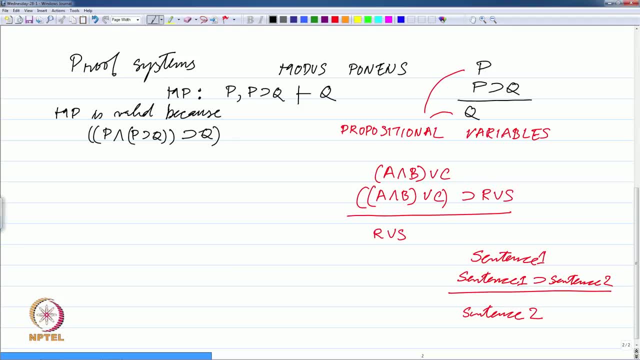 inference is based on a tautological implication. we had seen that in the last class. this is just a quick review of what we did recently. So what is the proof system? A proof system essentially does the following: that it is an algorithm. you might say that pick some rule, and when you say rule, we mean a rule. 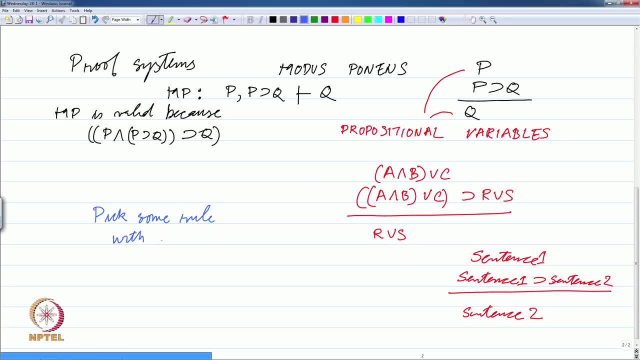 of inference with matching antecedents, which means in our knowledge base there are certain formulas which match the antecedents. Then add the consequent. So this is the rule of inference. 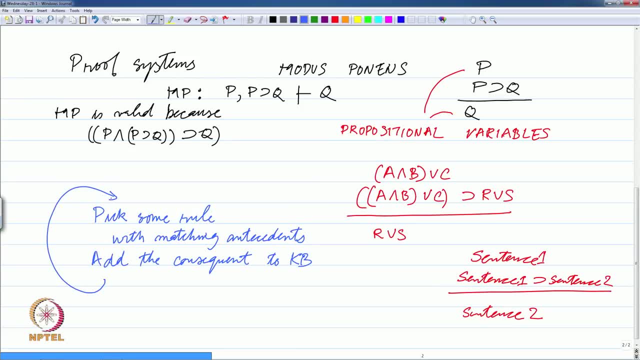 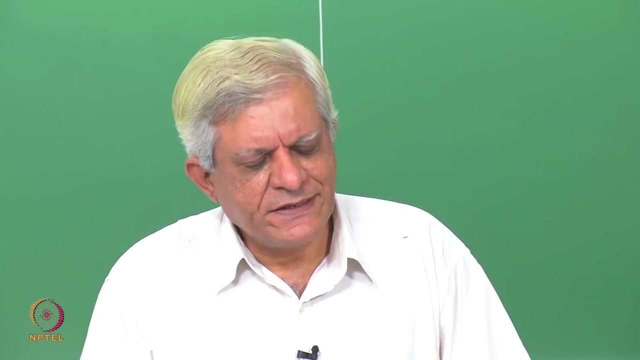 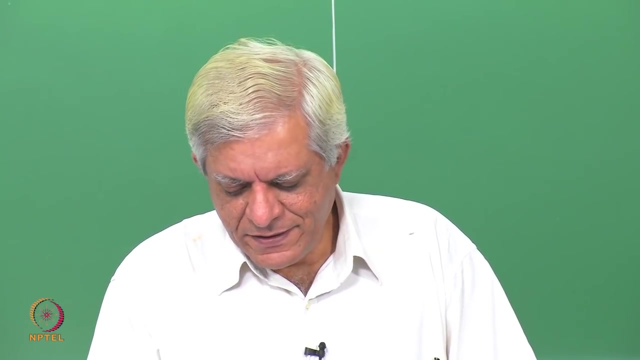 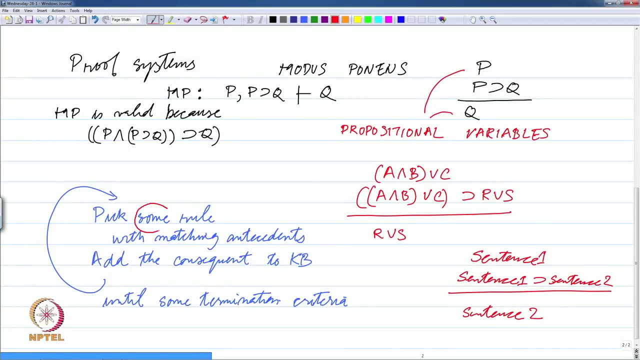 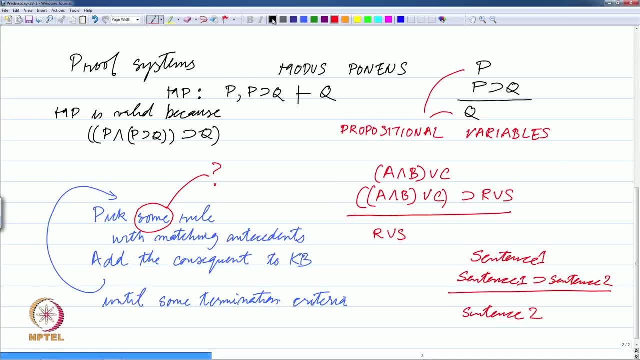 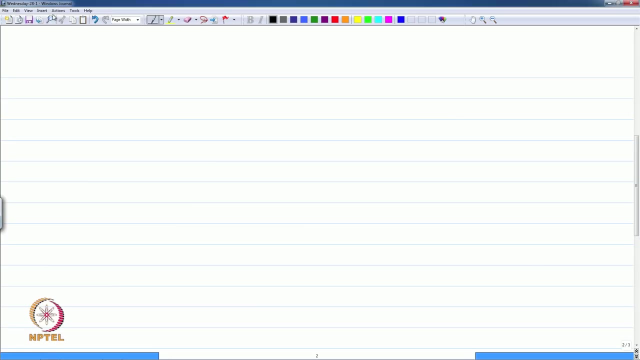 So that sum is going to be a very critical. So let us talk about the termination criteria. So by and large, we tend to distinguish between two kinds of proofs. One is called direct. 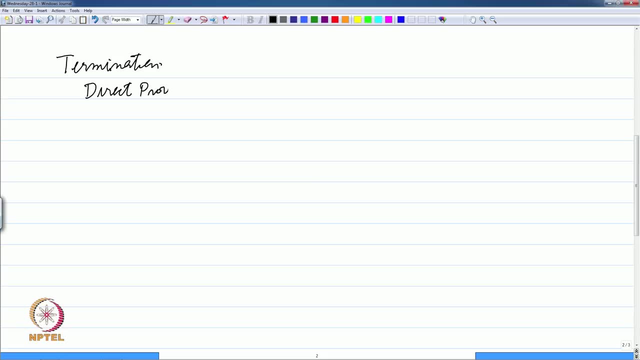 proof, or we use a term often, natural deduction. So we have thrown in the term deduction here. So at this moment we will simply say that deduction is that form of influences which use valid rules of influences And what we do in direct proof is the. 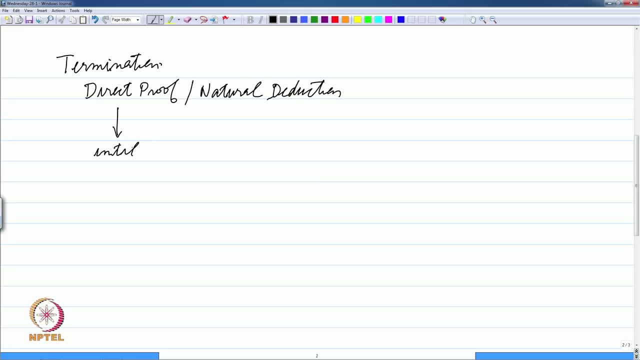 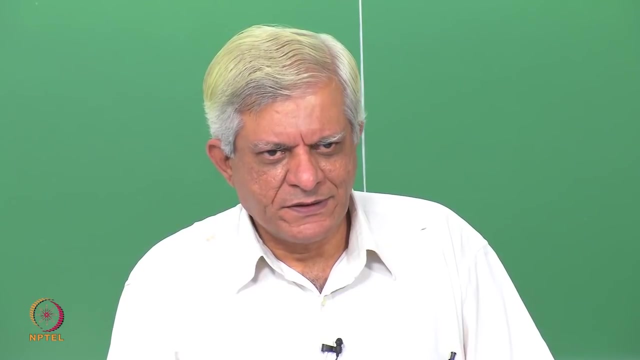 termination criteria is until alpha is added to the key v, where alpha is the sentence that you are looking for. You want to prove a certain statement And we use a term theorem In a direct proof. you keep adding formulas till you get the formula that you are looking for And that is the most natural form of proof And that. 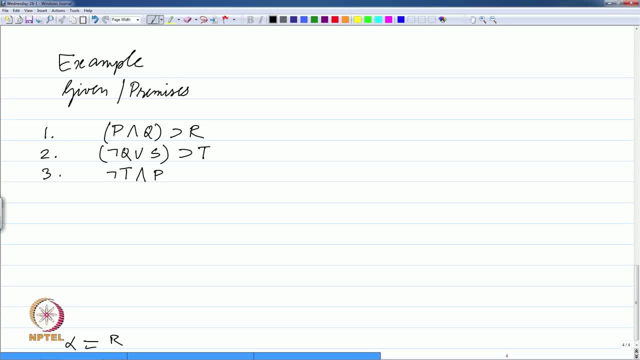 table. Just construct a large formula based on this and see whether R tends of the truth is not. but we are interested in proof methods right now, essentially, So let's do a proof of this. So for time, writing in blue, if you can make out our 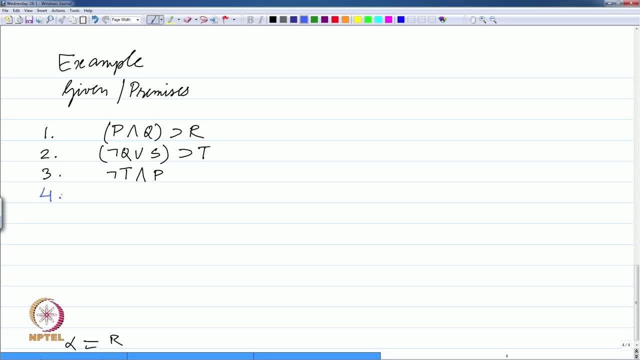 what I am writing in blue, if you can make out, are sentences that come out of this. So, for example, not t, So this comes So typically the way we write proofs are that: how did you get this not t? We got it from sentence 3. 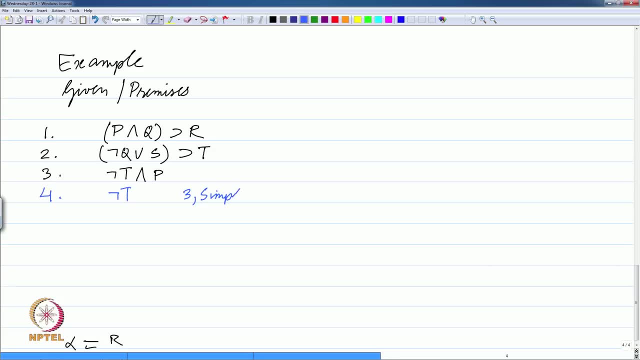 and a rule called simplification. You have to give a justification for every sentence So you can only use valid rules of inference. essentially 5, t, Again similar 3 and simplification 6, negation of not q or s. How do I get this? I get this from 4 and 2 and 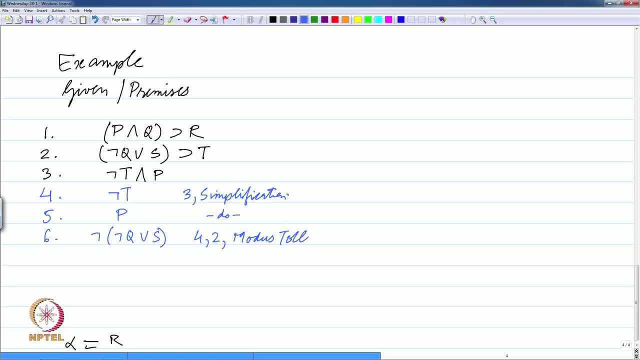 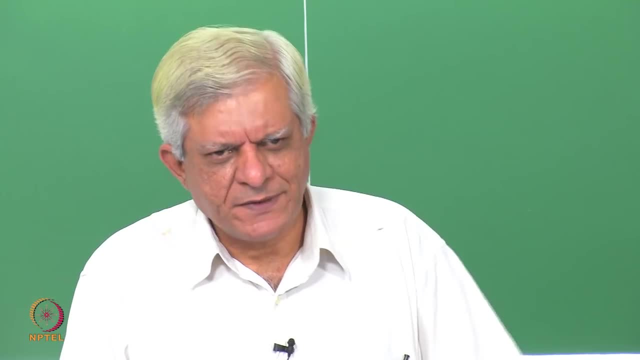 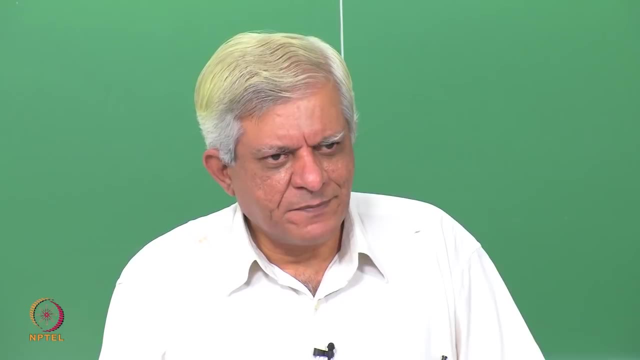 a rule called modus. It is one of the rules set. So, basically, a proof system will have a set of rules of inferences, and a lot of time was spent by logicians in trying to figure out what rules of inference do we need for a system to be complete. essentially, So, if you have more, 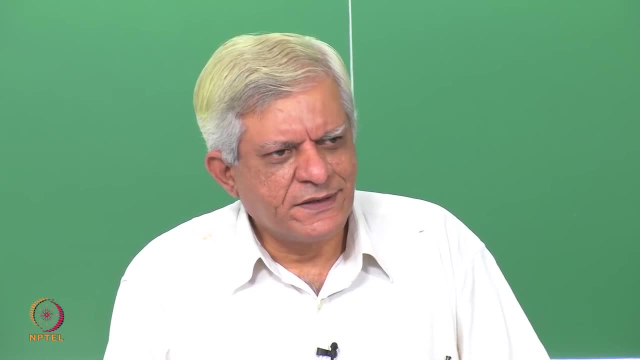 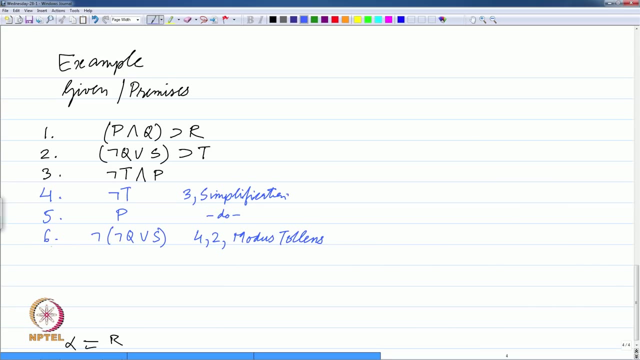 rules of inference. you can get possibly shorter proofs, but then the number of choices become larger at the same time. So there is a trade off between having more rules or less rules. anyway, Then we get this. So we push this inside. we get q and not and, which is from 6 and D. 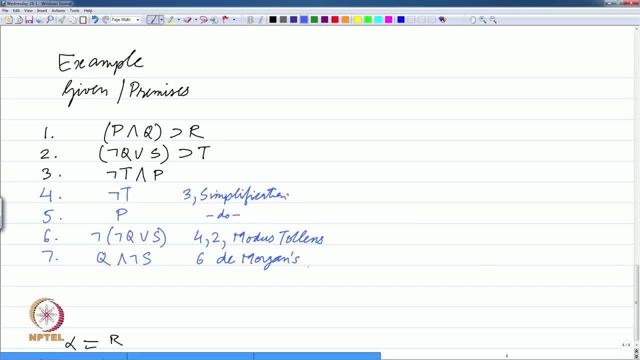 morgans, which I had not spoken about, but any text book and logic will tell you that you know When you push the not inside. I have skipped a step in which I said that 0, not q, should be q. essentially cool. From this I can get q. 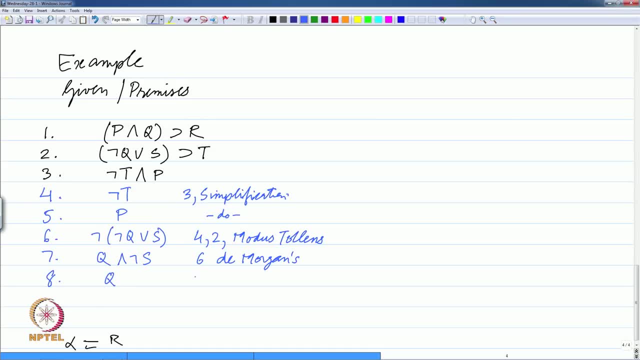 … which is 7, and simplification. then I can get p and q. So I get it because I have p, which is given in sentence 5, and I have q, which is given in sentence 8, and there is a rule called addition. And finally, I get r because I have 9 and 1 and our favorite, 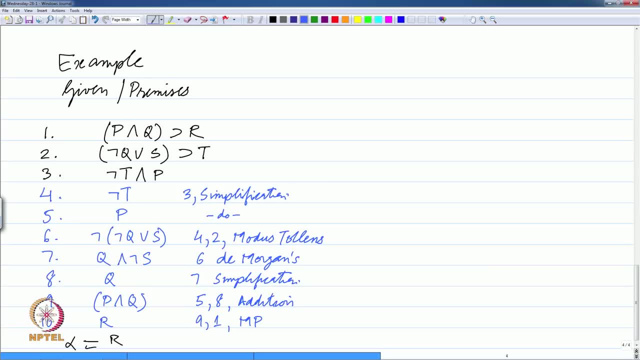 rule, which is modus ponensis, essentially. So I have managed to add some formulas to the knowledge base, So not t, then p, then other formulas, and in the end I added up, ended up adding a formula which is the. So this is the formula that we were interested in, which is r, essentially. So you can also 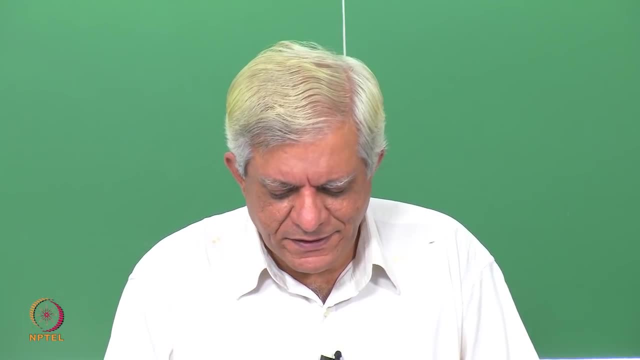 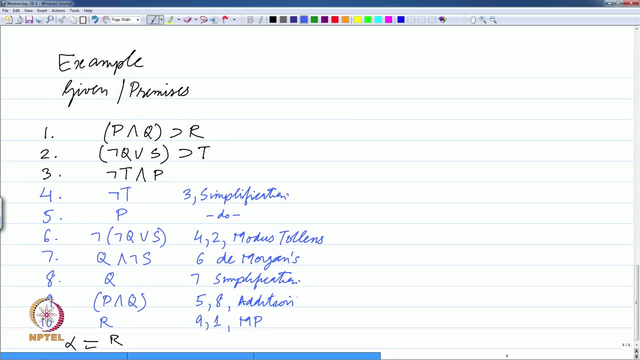 write this in a form of a tree, as I said, natural deduction tree. So, for example, at some point you would say that from this sentence and from this sentence I get r And the other things. you can actually construct the tree from those 3 sentences. you can. you know which? 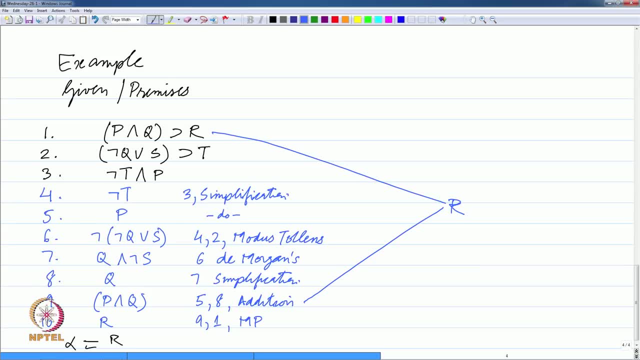 ends up with r as the. so this is a basic idea of a direct if you could get. Now, in this we assume that something was given to us And then from there we move forward. So one requirement of direct fuses: 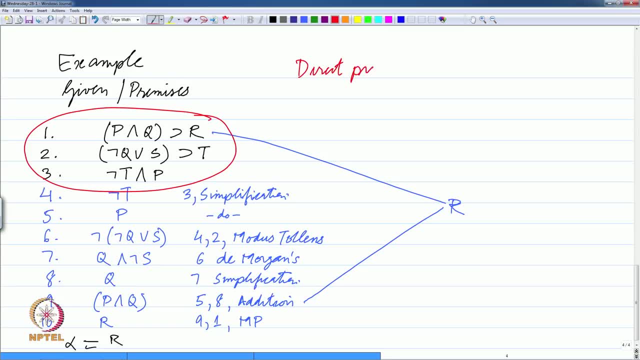 needs a set of starting sentences, because the, if you remember, the application of the rules is that pick some rule with some matching data. where is the? where is the matching data? it must be there in your knowledge base, essentially, So you must have. 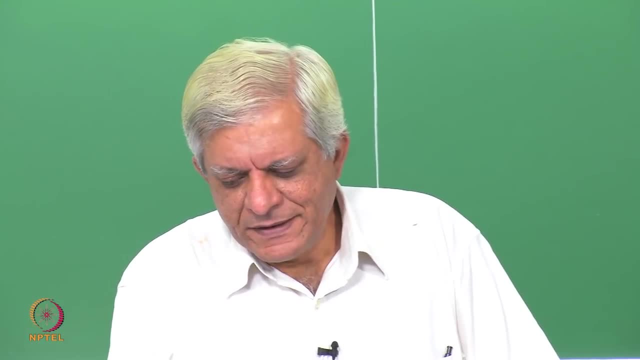 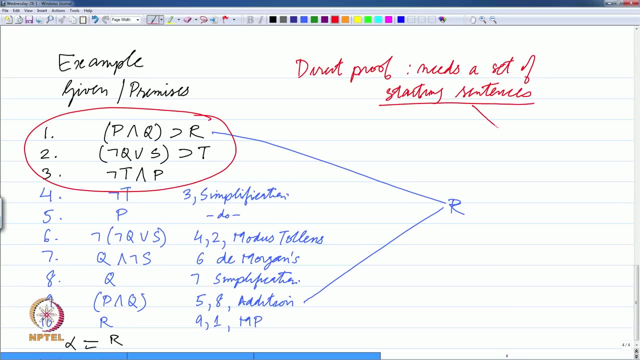 some knowledge base to start with, to which you can apply these rules. Now, there are two kinds of so these starting sentences. they are called axioms. by axioms we mean that, something that we, that something that we accept as true, and there are two kinds of axioms: one is logical and the other is. 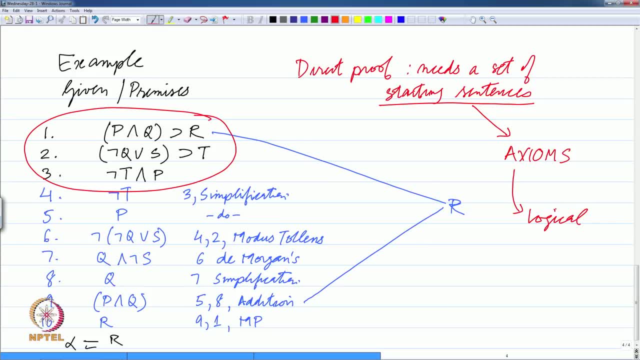 non-logical, which basically means that they are tautologies, and the other kinds are domain specific, which are given to us by the domains. So these domain specific axioms are the ones that we started off with here. essentially, we accepted these facts to be true because 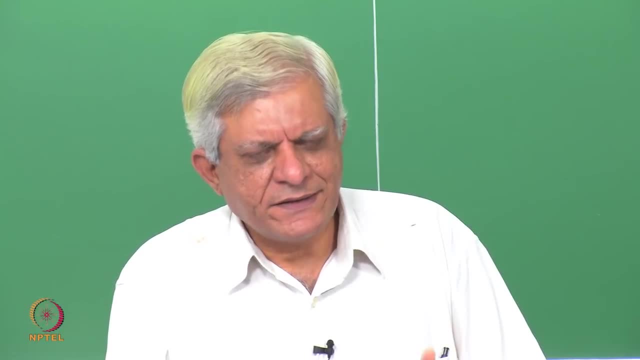 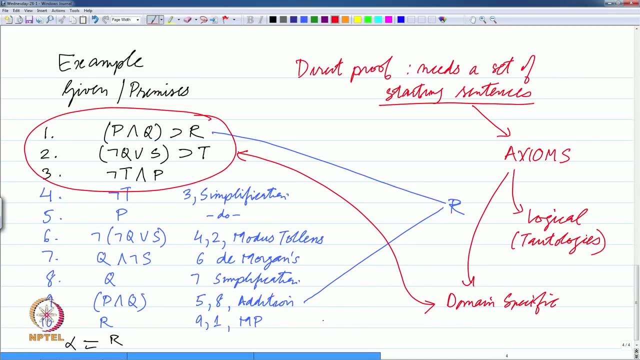 somebody said that this is true And in any case, we are interested in the entailment question. So what is the entailment question we are interested in? is that this set of sentences, which is, let me write here, p and q implies r comma naught q or s implies t comma. 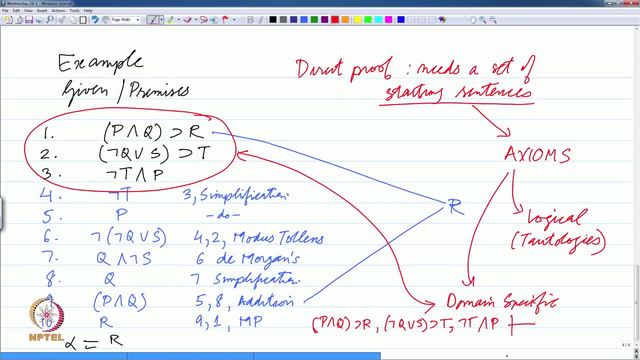 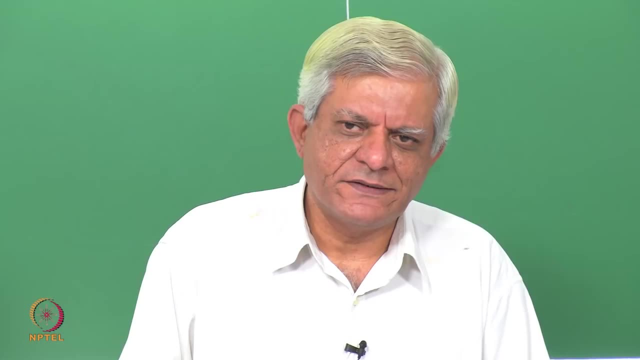 naught t and p entails r. this is the question that we were interested in. Of course, this is not entailment, this is derivation. but we are interested in those machines where the derivations will always correspond to the. We have said that we are interested in machines which are both sound and complete. 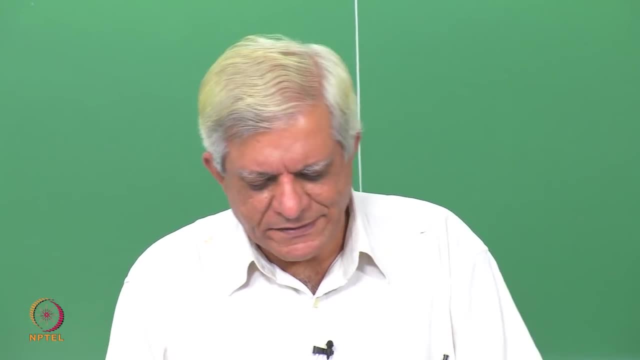 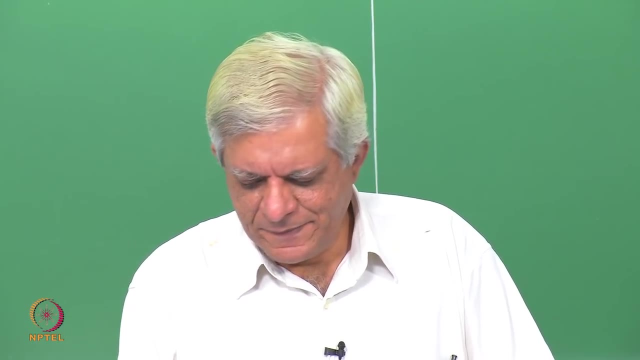 essentially So they if they produce. if my machinery produces r as it is done here, then it r better be true. otherwise what is the use of having such a machine? So we need a machine which is sound, essentially So. in the next class we will look at some of the early logical. 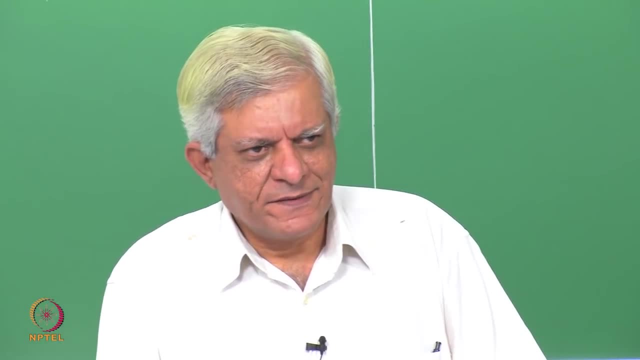 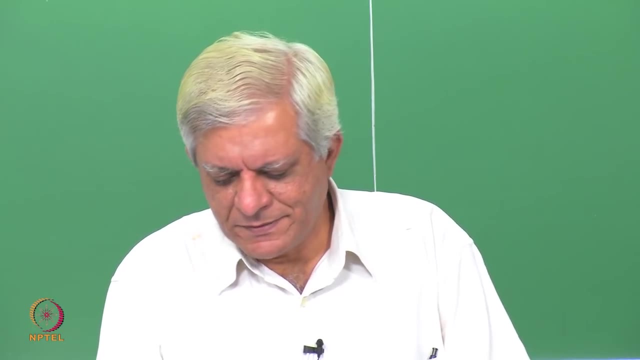 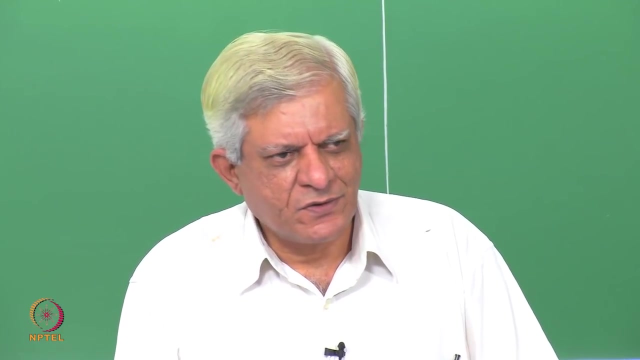 systems where the axioms for tautologies essentially, And then we will show that even working with domains with problems like this can be reduced to looking for tautologies. So that is why at the beginning of the class I said that we are interested in tautologies essentially. 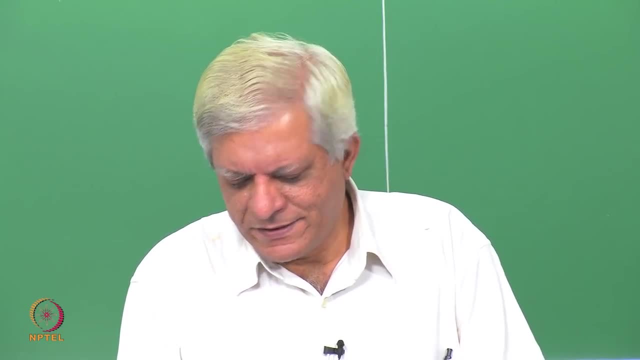 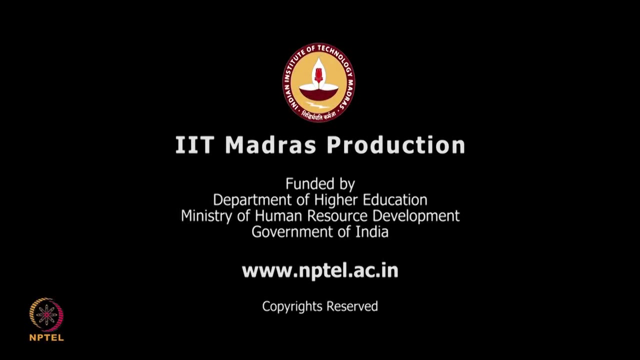 If you can solve, if you can find all tautologies. we can find problems like this essentially. So we will do that in the next class. Thank you,